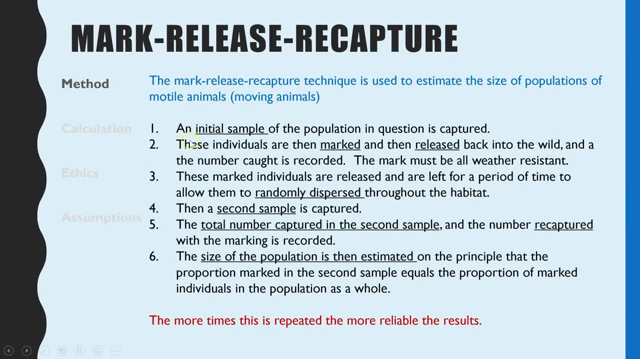 different bird species, for example. So the first thing you have to do, as the name of the method suggests, is capture an initial sample and you mark them. So the sorts of ways you might be capturing them would have to be ethical, so you're not causing any harm. It might be little pitfall. 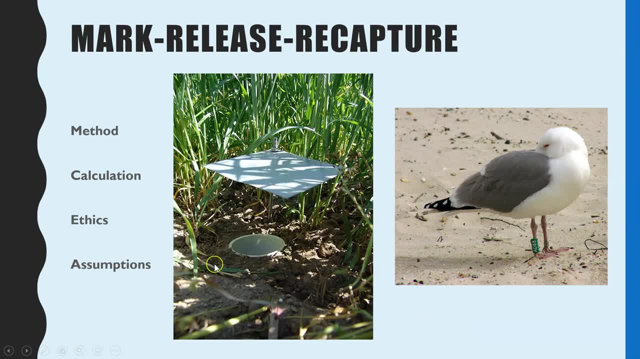 traps, which is what this diagram here is showing. So insects can crawl in, but they can't crawl out, and this shield here is to prevent excess water from getting in. So if you have a bird, that's water from dripping in if it rains, so they don't drown, Or for other animals it can be larger box. 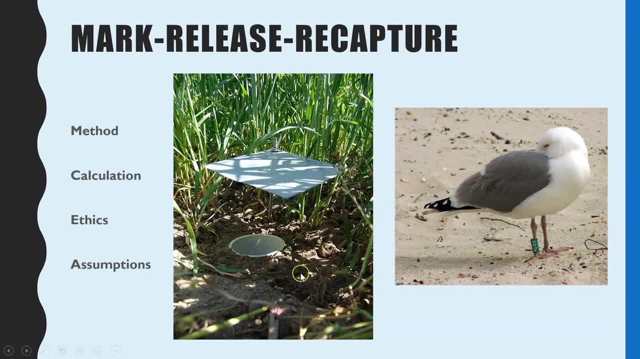 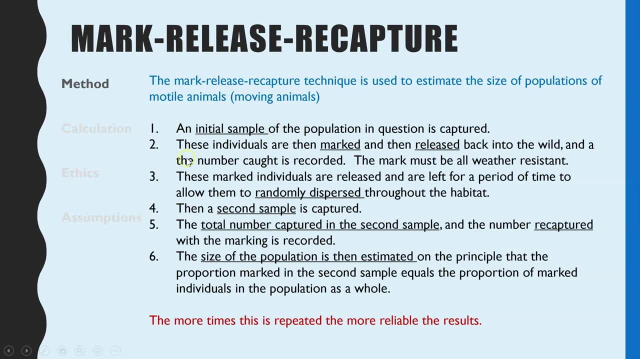 traps which shut when they enter and there's food and water provided inside for them. So that's step one. You need to capture an initial population, So you'd leave your trap set up for a period of time. you come back and then the individuals that you have captured, you would mark them in an ethical 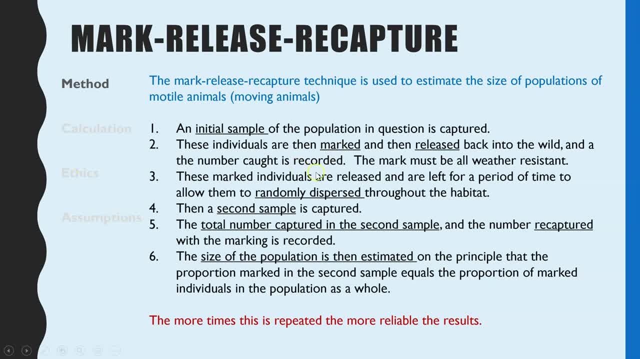 way, which we'll come to in the ethics section- And the mark that you put on has to be all-weather resistant, So it has to be something that is not going to wash off in the rain, for example. So once you've done that, you then release those animals. 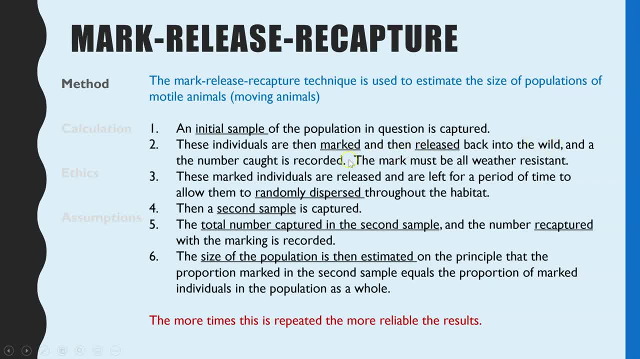 safely back into the wild and record how many you had captured. So that is the mark release part of the method. The next step is you need to leave those animals that you've released for a long period of time so that they should be able to randomly disperse amongst their natural habitats. 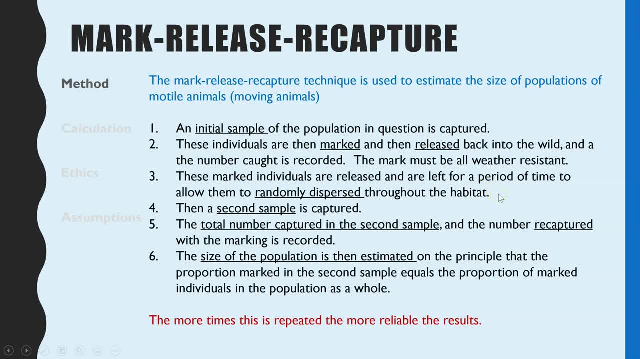 And that period of time will vary for each animal because it depends how quickly they move. Once you've left them for that period of time, you then set the traps up again and you capture a second sample. This time, though, you don't mark any individuals, we are just recapturing and you 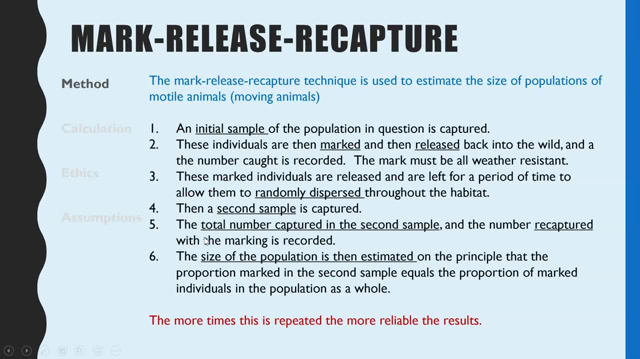 will need to collect certain data. collect is the total number that you have captured in your second sample, so you'd record that number down. you also need to record down from that sample how many of them are animals that were already caught, which you know because they are marked in some way. so you are recapturing, counting the total. 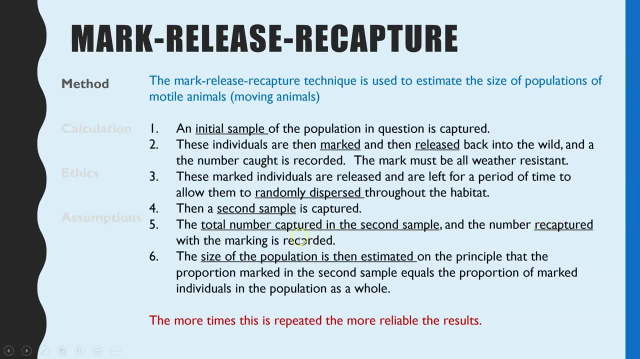 number in your sample and, within that sample, counting how many have the marking on. you're then going to use this data in the calculation to come up with an estimate for the size of the entire population. so this is the sampling technique. you're not counting every single. 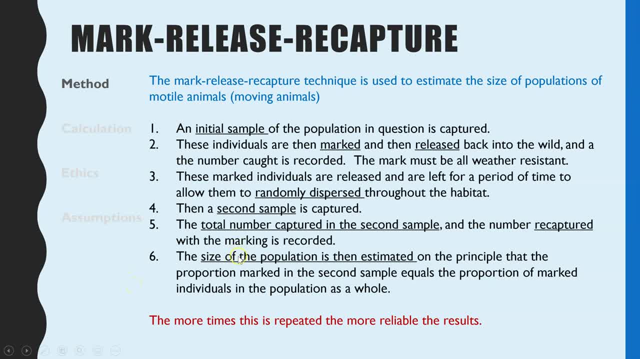 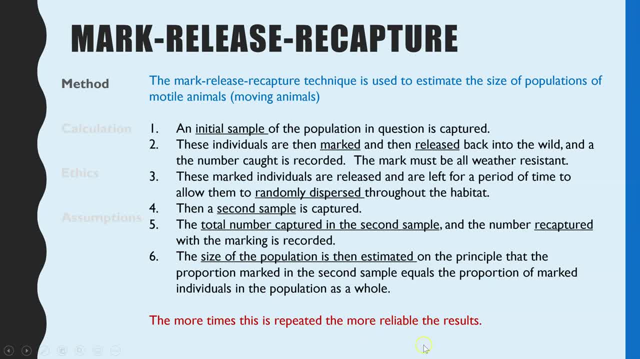 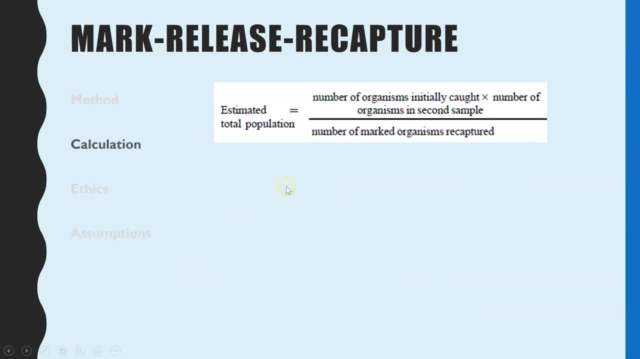 calculate a mean, you would get more accurate and reliable results. so you should do multiple repeats, so the calculation. then let's have a look at how we'd actually use that data. you do need to know this calculation for aqa, for a level they wouldn't provide you with this and in an exam 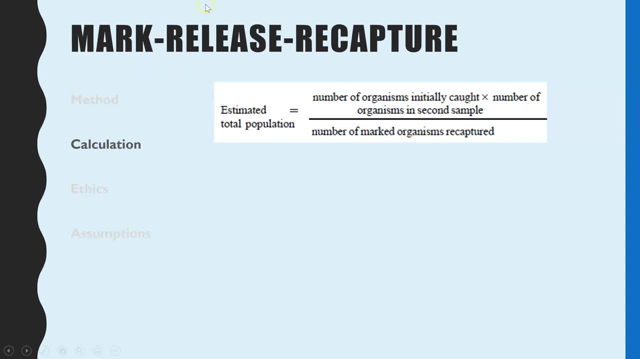 question, where it might be a long answer question, and they ask you to describe and explain the method. there would be one mark just for stating this equation, so to calculate your population. this is how we then use all the values we collected, the number of organisms that you 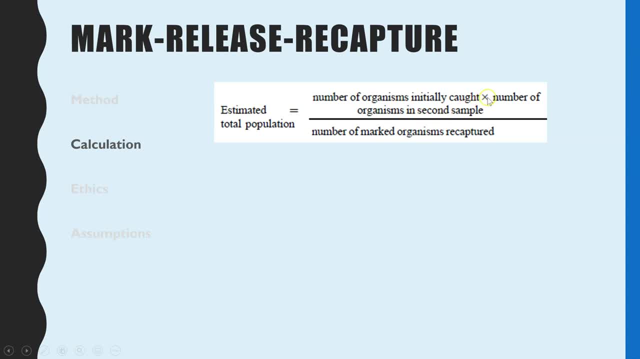 initially caught um, and then that would be multiplied by the number of organisms in the second sample that you caught, divided by the number of marked organisms recaptured. so just to go through an example, let's say i've been sampling a particular butterfly species. in my initial capture i caught 20 butterflies and i marked all of them. i then released the. 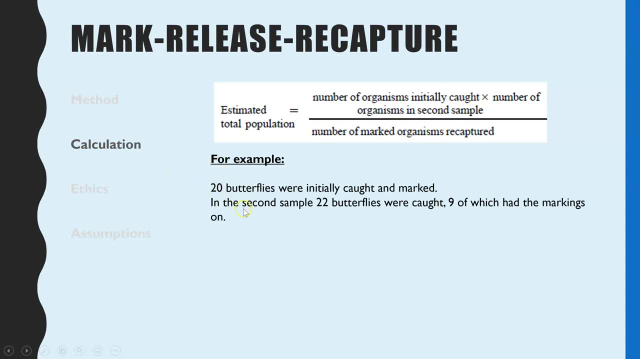 number of organisms, and i took the second sample and this time i captured or recaptured 22 butterflies, but i recaptured nine because out of those 22, nine were marked. so that would mean i'd be doing the number of organisms initially caught, which was 20, multiplied by the number of 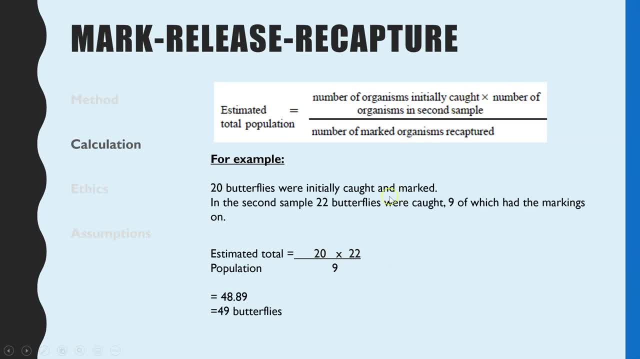 organisms in the second sample, which was 22, divided by the number of marked organisms and of marked organisms recaptured, which is nine. So in this example my sampling mark release recapture method would give me an estimate of 48.89. but because we're talking about animals, you do have 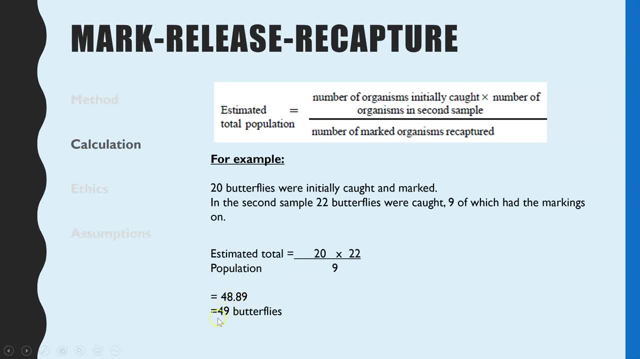 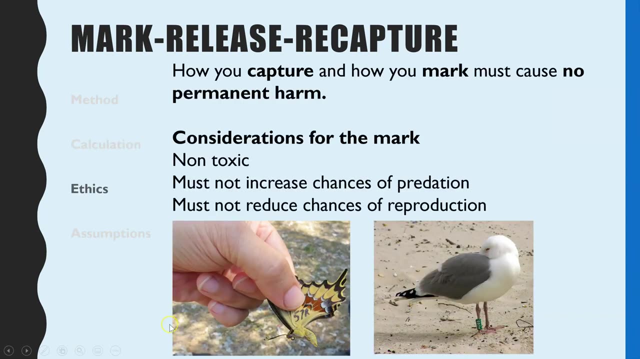 to round up or round down. so I'm going to be rounding up in this case and I'd be estimating that in that particular habitat there are 49 of that butterfly species. So that would be our estimate of the population. So, thinking about the ethics, this is a key thing with sampling animals. 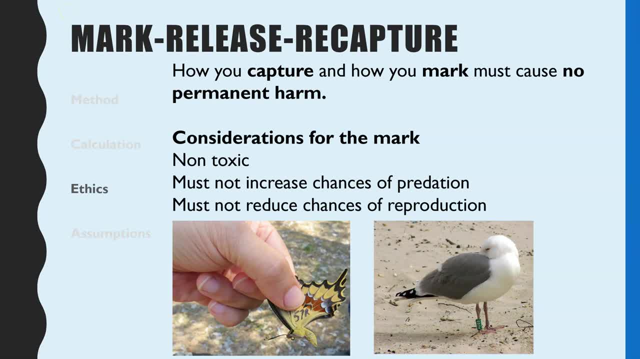 So the main thing you need to be aware of is not exact techniques of how to be ethical, because you would have to know so many different methods. it'd be too extensive. What you have to know, though, is that whichever method is chosen to capture and to mark, the animal has to be ethical. 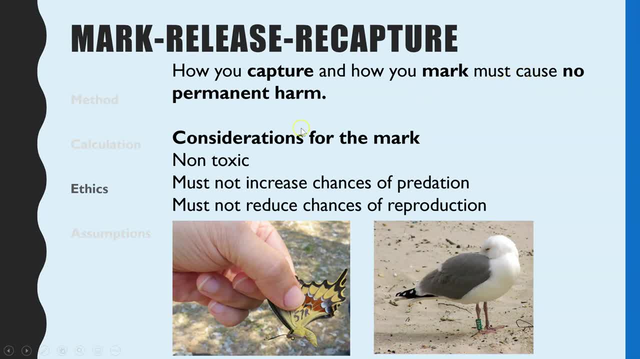 and what we mean by that is it has to be a method that causes no permanent harm or pain to the animals. So if you were asked how to sample or how to capture bees ethically- that did come up in one of the exam questions- you don't have to give an exact technique of how you'd do it. you would just say you would choose. 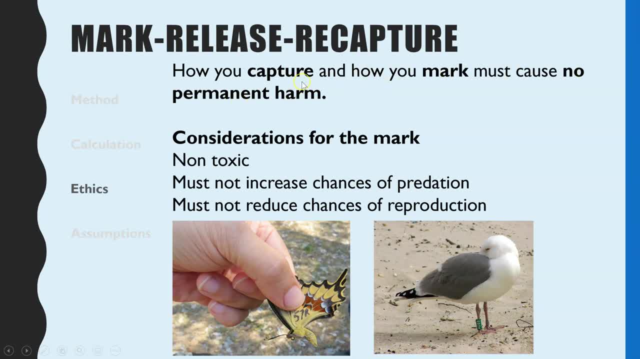 a method that causes no permanent harm. So that's how you'd capture them ethically. For the mark, there is a bit more detail of what you'd need to say when you consider how you'd tag the animal. So if you were asked how to capture bees ethically, that did come up in one of the exam questions. 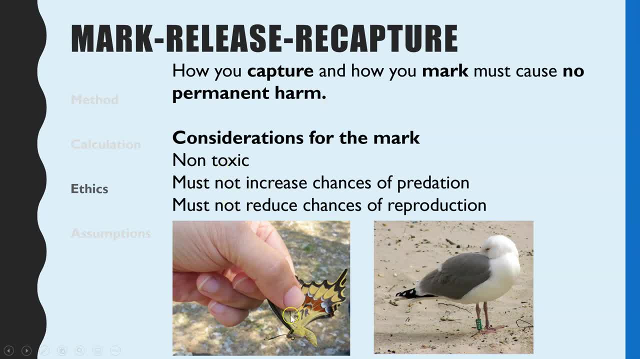 tag the animal or mark them. So, number one, if you're going to be painting on a tag so we can see that on this butterfly they've painted on a particular number as a tag, the paint that you use has to be non-toxic. it has to be all weather resistant as well, but that's not ethics, that's. 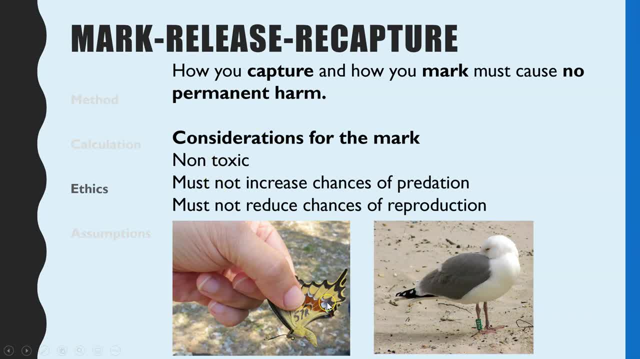 practicalities. You also have to make sure that the paint that you're adding on, or if it is a physical tag, like this one around the bird's leg, it must not increase their chances of predation, So it can't be some bright colour that will then interrupt their camouflage, for example. It also 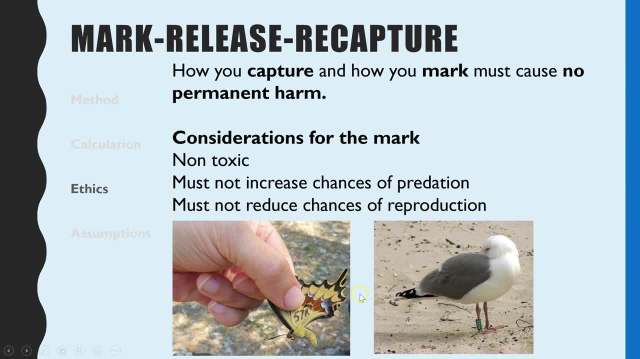 must not reduce their chances of reproduction, so it shouldn't interfere with their courtship ritual. Other things to consider. so this tag here on the bird isn't interrupting their ability to fly. so you've got to make sure that whatever you are doing to mark the animal, it's not toxic, it's. 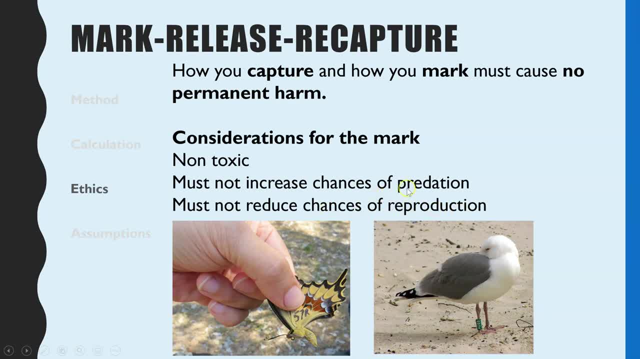 not going to harm them, doesn't interfere with reproduction and it doesn't make them more obvious to people. So if you're going to be painting on a tag, you've got to make sure that it's not going to cause any harm to predators. So the last thing you need to know about the mark.